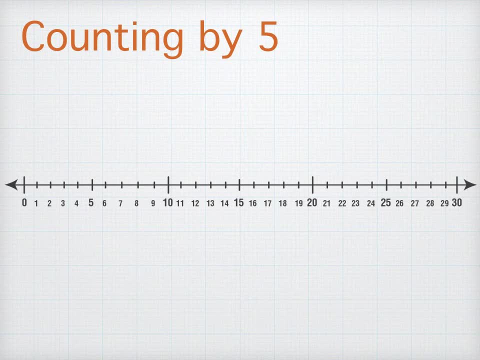 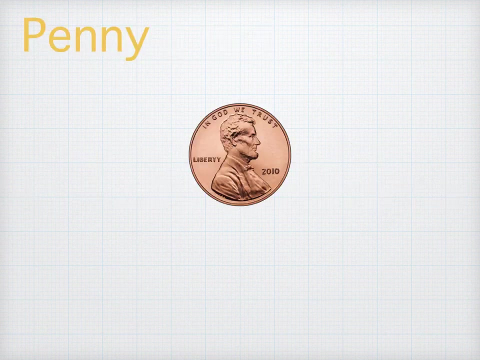 Before we begin counting money, let's review counting by 5.. Counting by 5 means we count up in increments of 5.. On a number line, that means we start at 0 and move to 5,, then 10,, then 15,, then 20,, 25, and so forth. 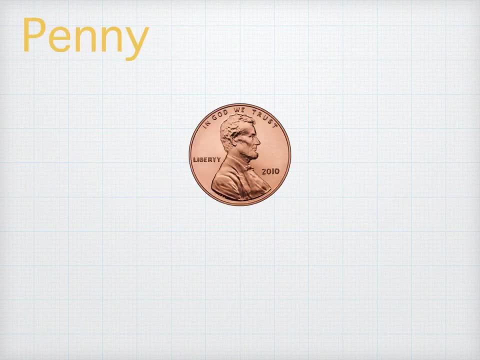 When using touch math to count pennies, we simply draw a line and that line represents 1.. So with this penny, I draw a line and we have 1.. The unit for change is cents, so this means I have 1 cent. 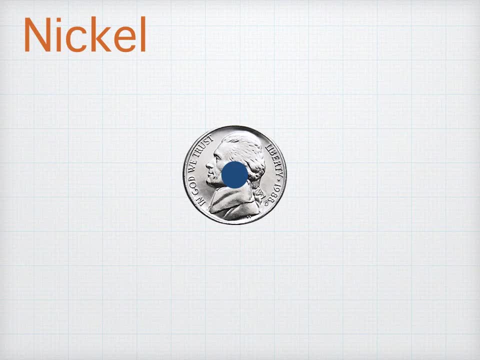 When using touch math to count nickels, we count the points. Each point is worth 5.. With a nickel, I touch my pencil to the point and count 5.. The unit for change is cents, so this means I have 5 cents. 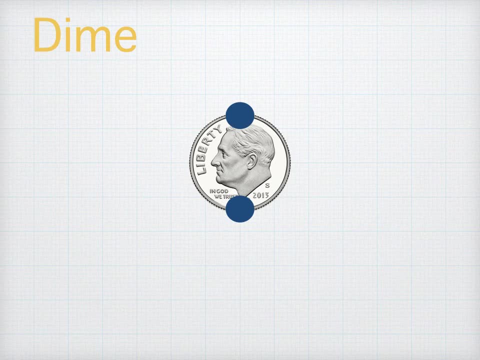 When using touch math to count dimes, we count each of the two points. Again, each point is worth 5.. So I have 5, 10. This means I have 10 cents. When using touch math to count quarters, we count each of the points. 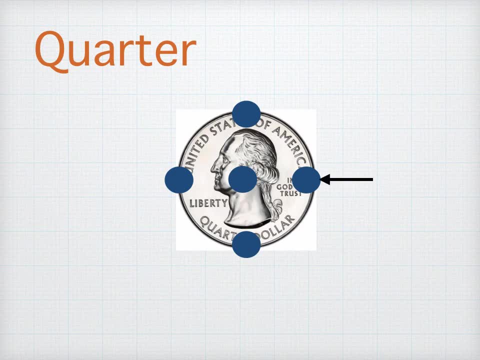 Again, each point is worth 5.. So I have 5,, 10,, 15.. 20,, 25.. Again, the unit for change is cents, so I have 25 cents. Now that we know what each coin is worth, we are going to practice counting change. 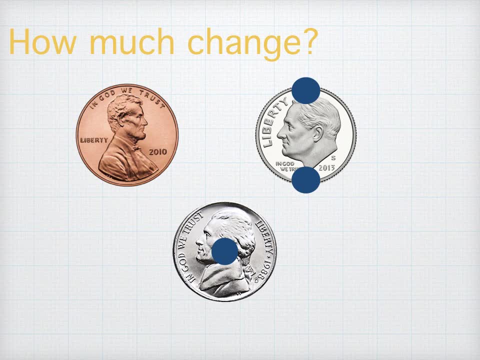 In this case, we have a penny, a nickel and a dime. How much change do we have? We will start by counting the dime, So 5, 10.. Then we will move on to the nickel 15.. And then the penny is last. 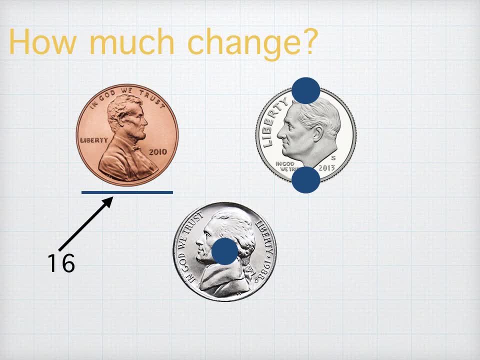 The penny is worth 1.. So we have 16.. This means we have 16 cents. Remember these points are different than the points for counting. When we count, each point is worth 1.. So 1,, 2,, 3,, 4.. 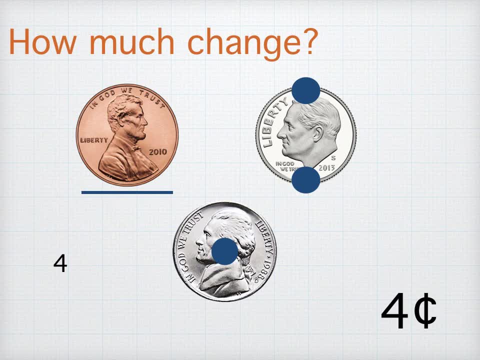 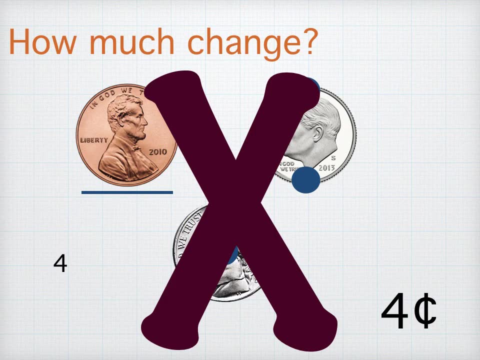 This is not the same for counting change. You do not want to count 1,, 2,, 3,, 4.. That is because each point is worth 5, except for pennies that are worth 1.. Touch math can help us count change, but we must remember a few rules.